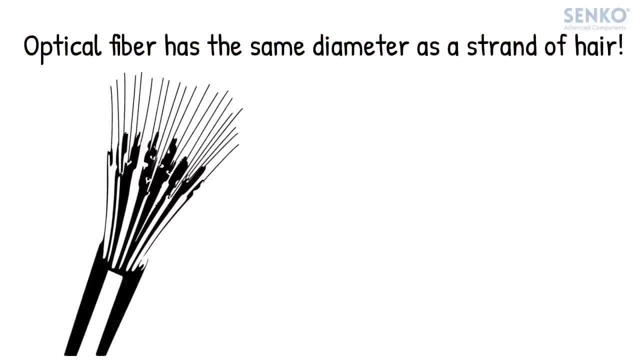 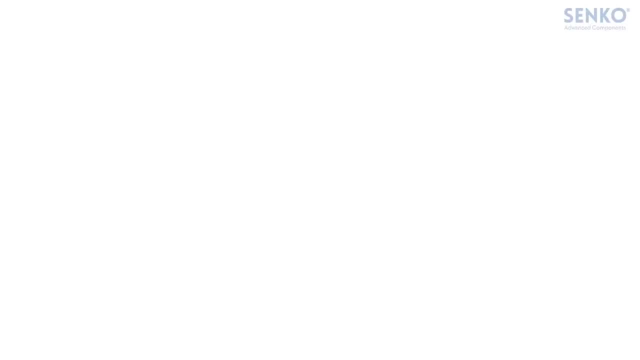 Basically, an optical fiber is a very thin strand of glass about the same diameter as a strand of hair. Pretty impressive, isn't it? To the naked eye, all optical fibers may look the same. however, that's not the case. There are many different types of optical fibers. 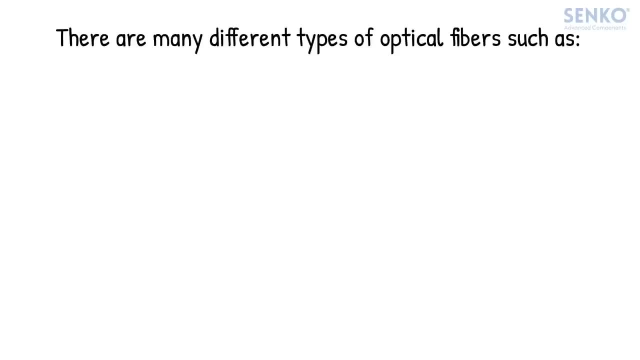 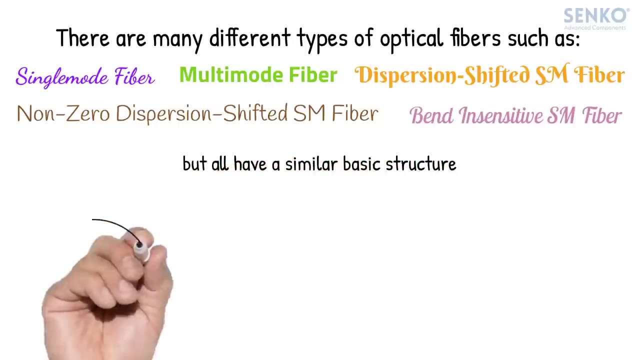 each with their own specific application. Some examples are the single-mode fiber, multi-mode fiber, dispersion-shifted single-mode fiber, non-zero-dispersion-shifted single-mode fiber and bin-insensitive single-mode fiber. All of them have a similar basic structure. 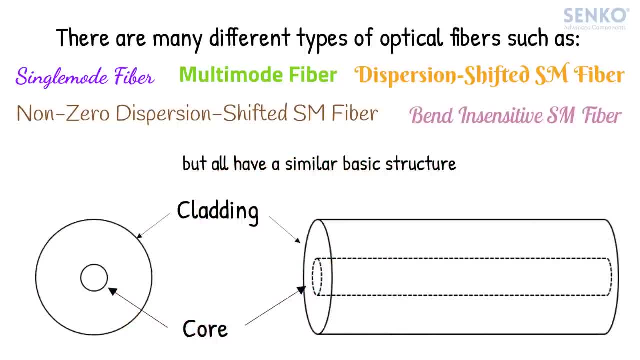 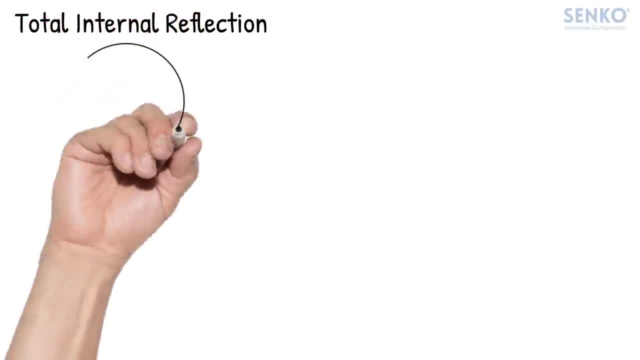 which is a core in the middle and a cladding around it. The fiber core and cladding have different indexes of refraction. This difference keeps the light from escaping the core through a phenomenon called Total Internal Reflection or TIR. Generally, there are two types of optical fiber, namely the single-mode fiber and 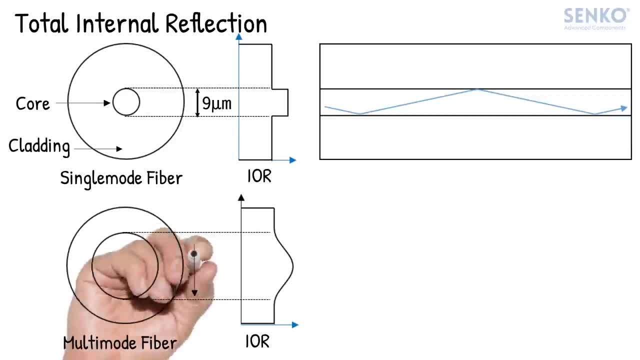 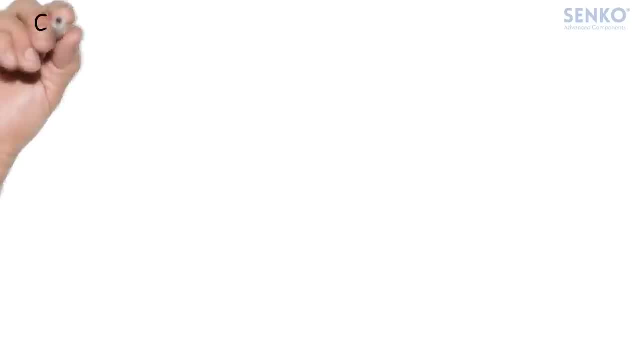 the multi-mode fiber. They have different core sizes and index of refraction which make light behave differently inside of the core To the naked eye. all optical fiber has the same: single-mode fibers and multi-mode fibers can further be broken down to different categories. 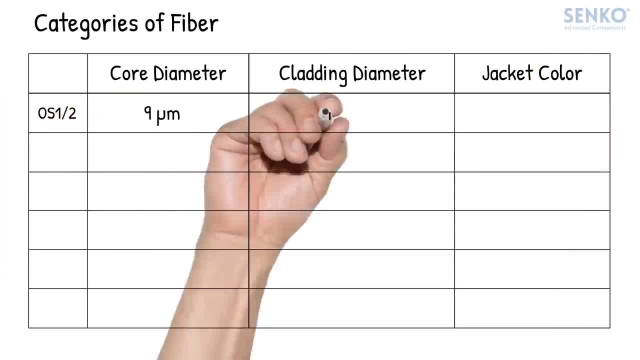 The single-mode fiber can be categorized under as OS-1 and OS-2. While both have the same physical dimensions, OS-1 fiber has a higher attenuation per kilometer of fiber and is only suitable for indoor use, while OS-2 fiber is suitable for indoor and outdoor deployment. There are five 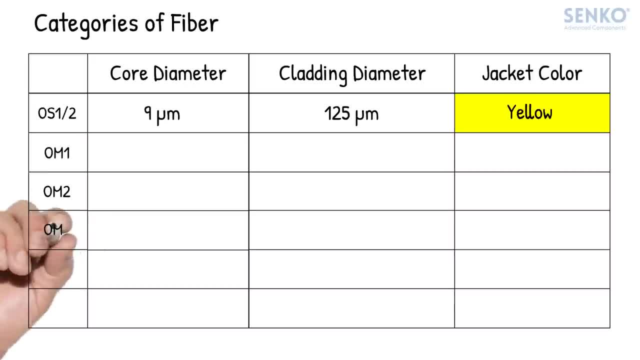 types of multi-mode fibers, which are OM-1,, OM-2,, OM-3,, OM-4, and the OM-5.. With OM-1 being the oldest standard and OM-5 being the latest, they have different core diameter sizes. 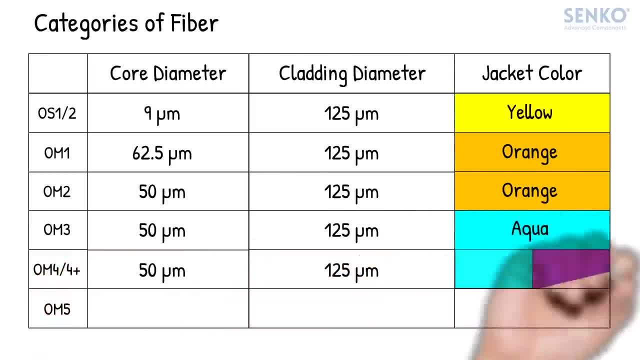 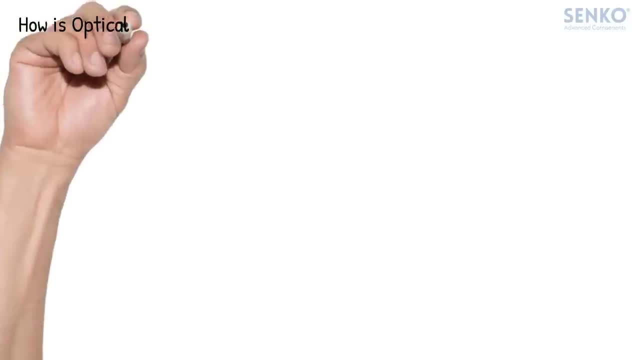 and can commonly be identified based on the standard jacket color defined by various standard bodies. Each type of multi-mode fiber has a minimum modal bandwidth, with the latest multi-mode standard OM-5 being able to support higher bandwidth transmission for longer distances compared to the earlier standards. 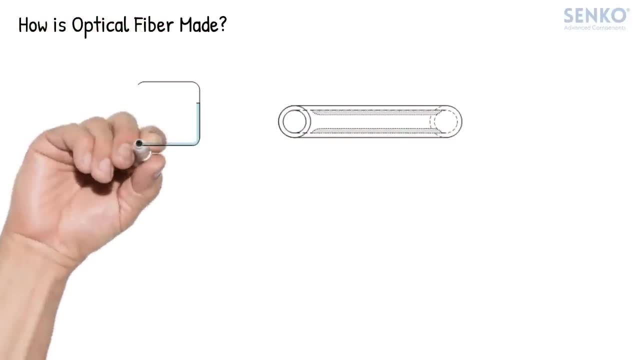 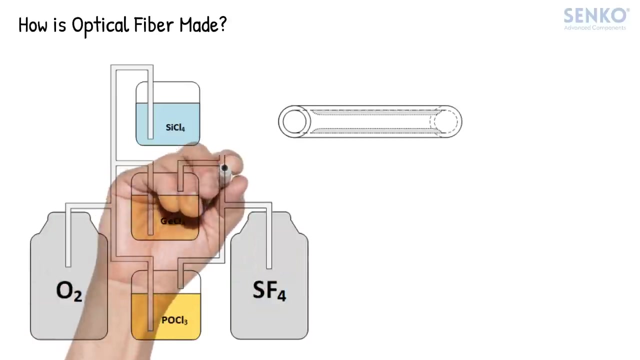 Optical fiber starts as a hollow tube of glass. Gases that contain silicon, germanium and many other chemicals are injected through the rotating tube. The glass tube is then heated by an oxyhydrogen burner that traverses its length. This creates soot deposition on the inner wall of the glass. 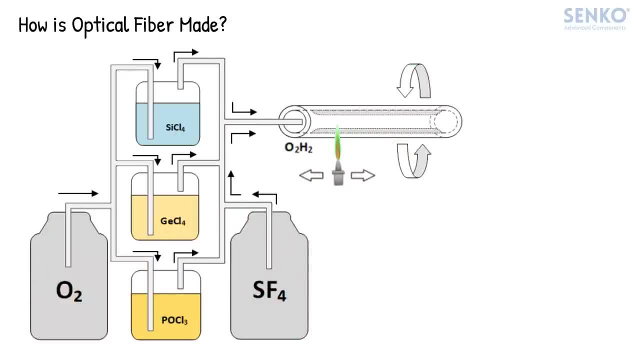 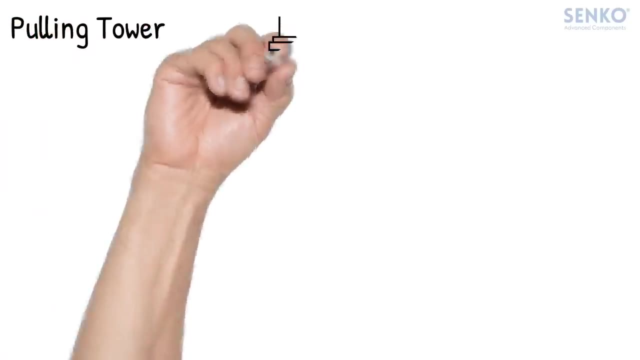 tube. Further heating at higher temperatures during rotation causes it to collapse uniformly, which results in the production of a fiber preform. A fiber preform is a rod of pure glass with a refractive index identical to that of the desired fiber. The fiber preform is then mounted at the top of a pulling tower which feeds it. 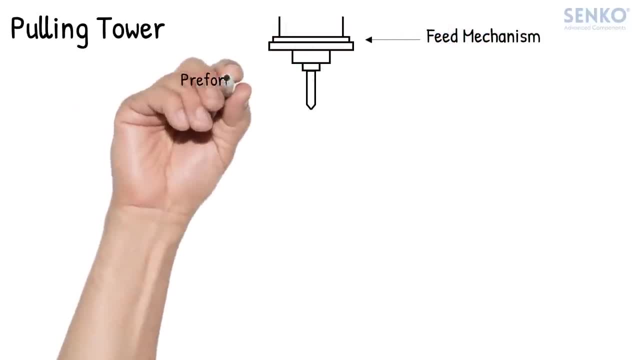 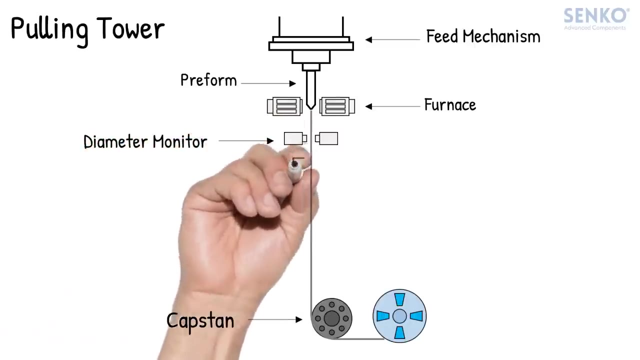 through a furnace that heats the bottom of the platform until it starts to melt. The melted fiber preform then drops, with the help of gravity, down to a capstan where a constant tension can be applied on the optical fiber. As more melted fiber preform is pulled, it is monitored to ensure constant. 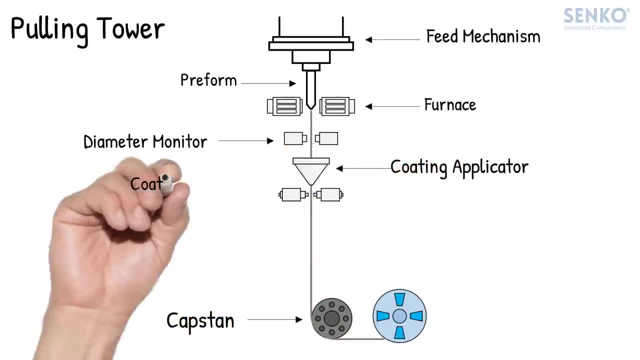 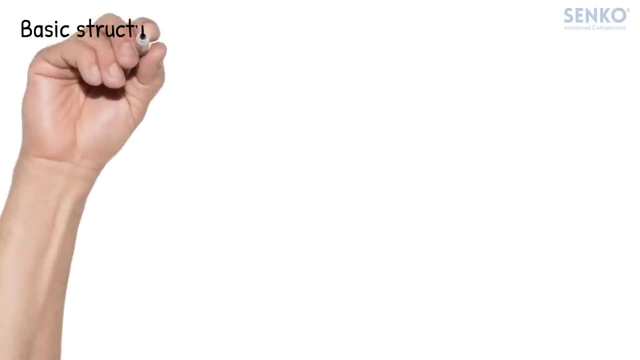 diameter within the acceptable range. An acrylic coating is then applied and cured for added protection and color. for identification, The fiber is then coiled onto a fiber spool ready to be used to manufacture different types of fiber optic cables. Let's have a look at the makeup of a standard optical fiber cord. 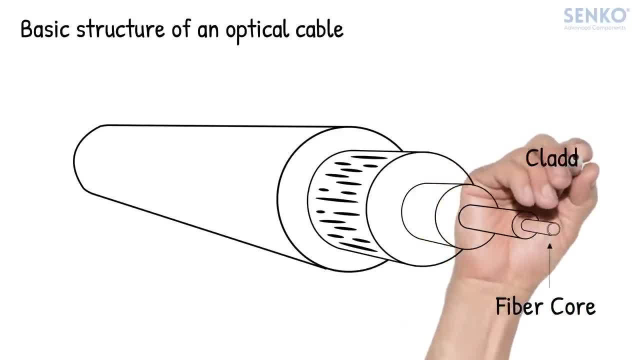 We start off with a strand of optical fiber with a layer of cladding. The cladding is then oversleeved with an acrylic coating. Aramid yarn is then layered around the assembly to increase the tensile strength of the cord. The whole assembly is then protected with an outer cord jacket. that is. 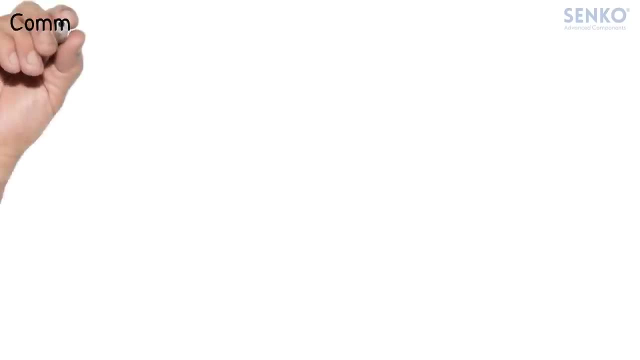 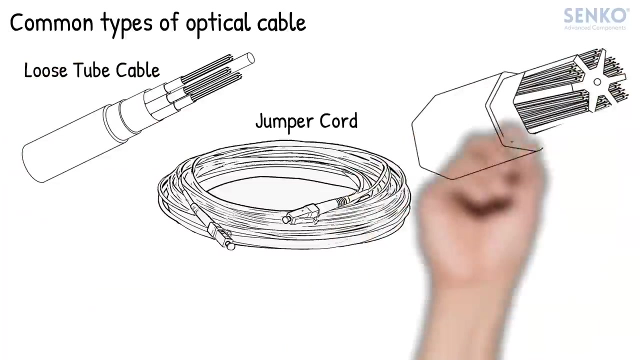 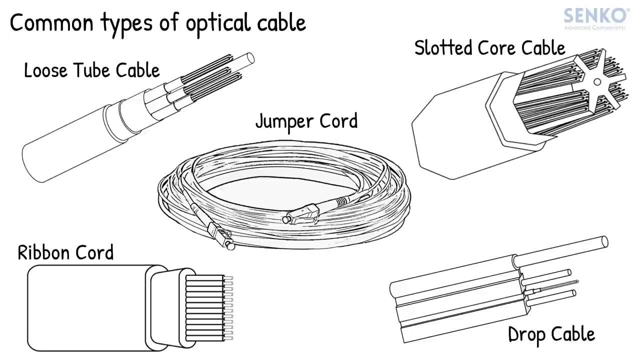 usually made with polyurethane or PVC. Other than fiber cords, some other fiber cable construction deployed around the world are the slotted cord cable, drop cable, ribbon cords and jumper cords. Instructions are constantly changing to increasing market demands and requirements for deployment. 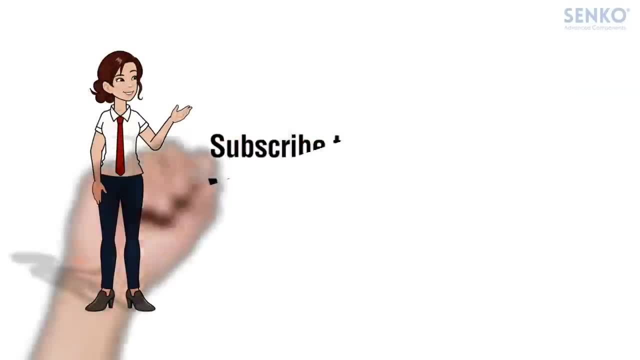 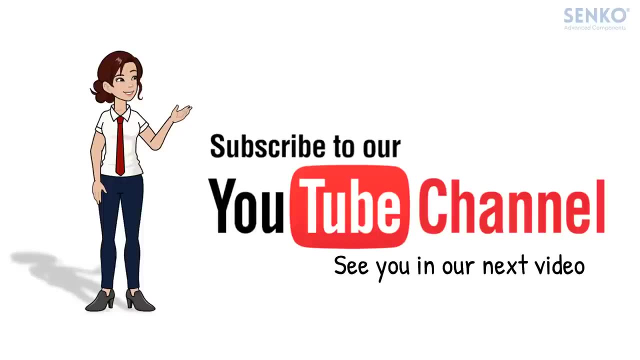 Well, that's all the time we have. We hope that you were able to learn something about the various types of optical fibers and how they are made. Please like and subscribe to our YouTube channel for the latest updates, and we will see you in our next video. you.